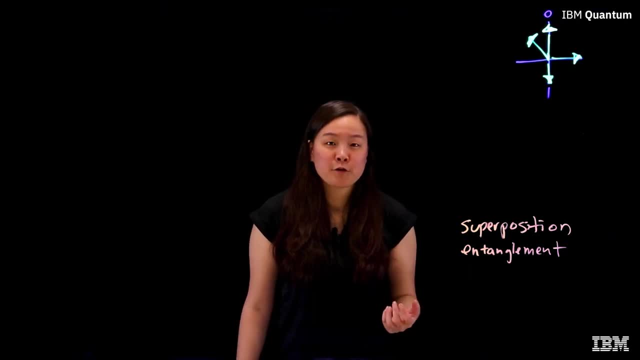 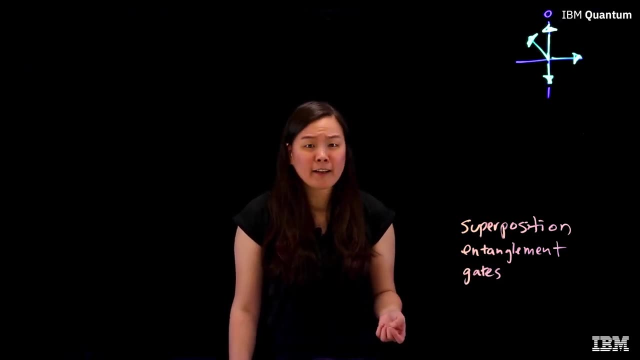 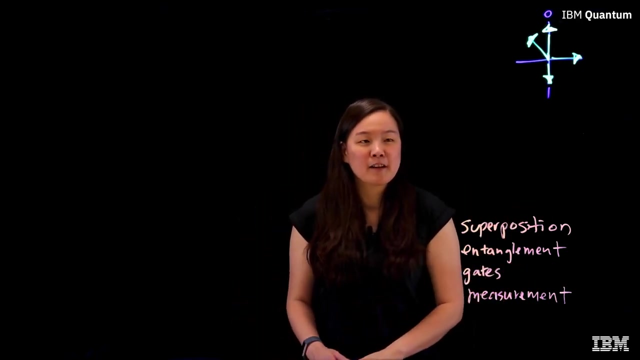 states become strongly correlated. In order to change the states of a qubit, we apply a series of gates, similar to the classical logic gates, And in the end we want to match these qubits so we can get the results. So how do we take all these concepts into code? And the answer is simple: We use a quantum. 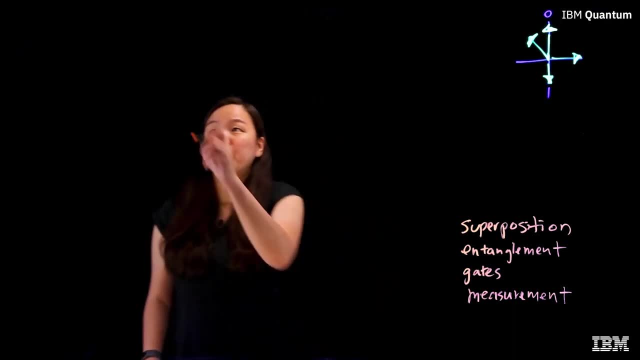 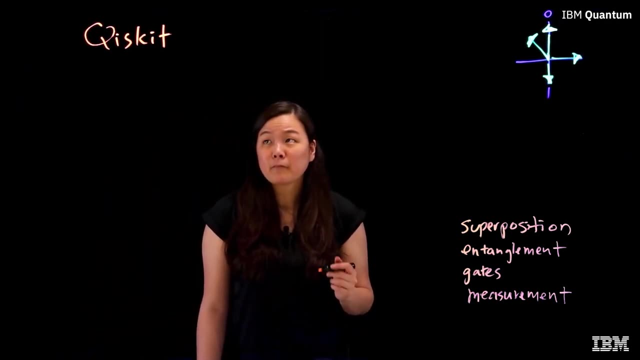 software development kit. In this video, we will be using Qiskit, which is the most widely used quantum SDK today. Qiskit is based on Python, which is fairly simple to learn, even if you've never used it before. So let's write a simple program in Qiskit. 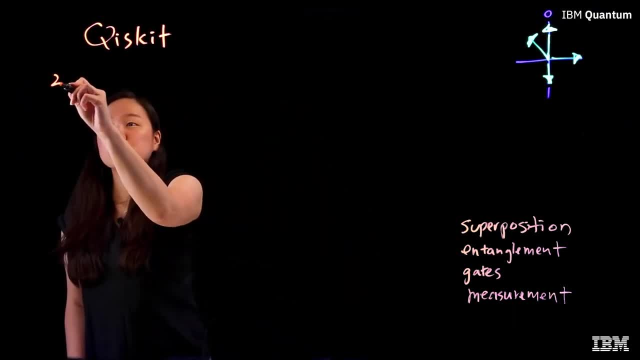 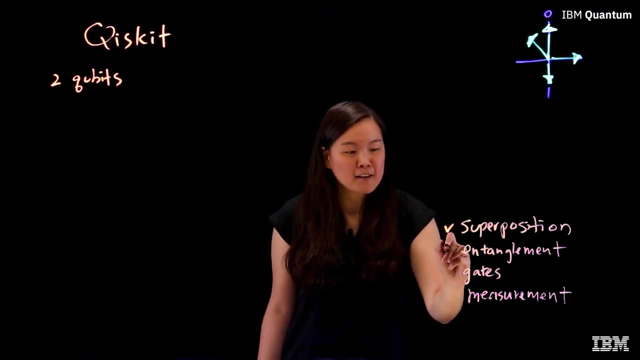 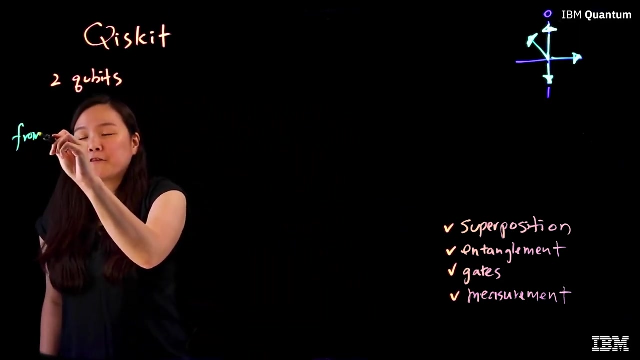 In this program we will use two qubits. We will put one into superposition, entangle it with the other and then do a measurement of both of them. And of course, OLA is done using gates. So let's start by importing Quantum Circuit from Qiskit. 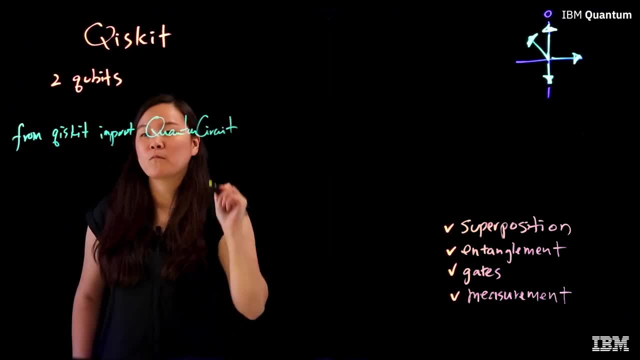 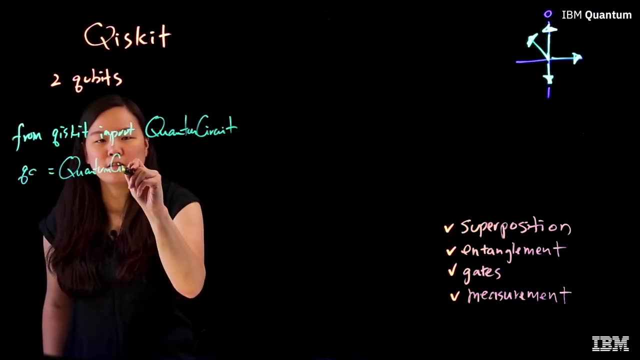 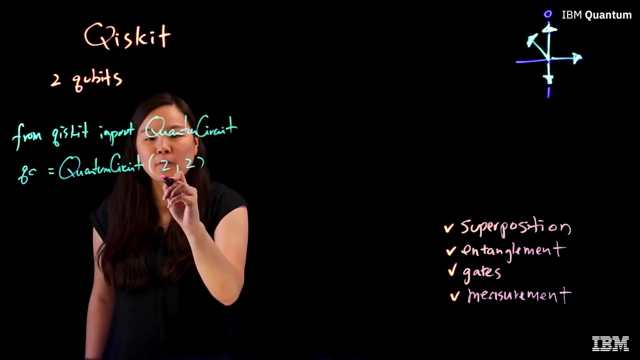 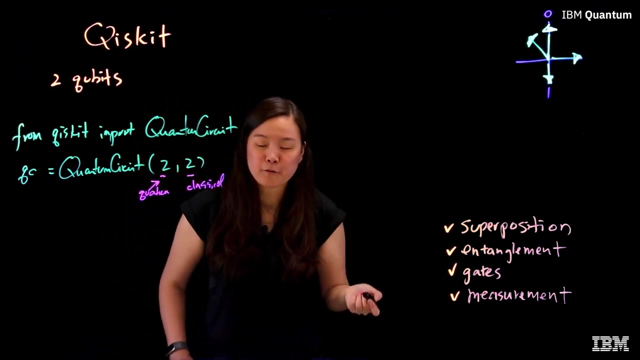 We then can create a quantum circuit with two quantum registers and two classical registers. The quantum registers are used for quantum computation, one for each qubit, and the classical registers are used to store the measured results. We need the classical registers because, even though the physical world is quantum, the 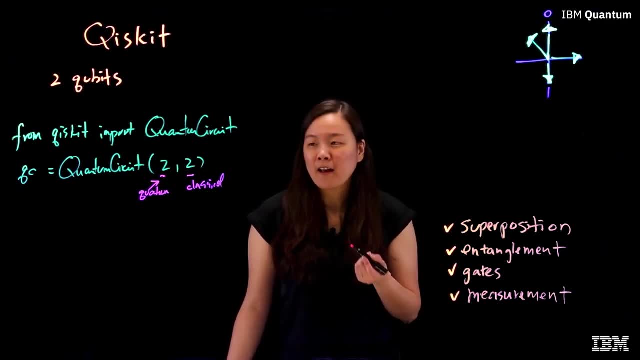 majority of the classical world is still classical and the classical registers allow us to bring the quantum information back into the classical world. So the next thing we want to do is apply some gates, and in this program we're going to apply two gates. 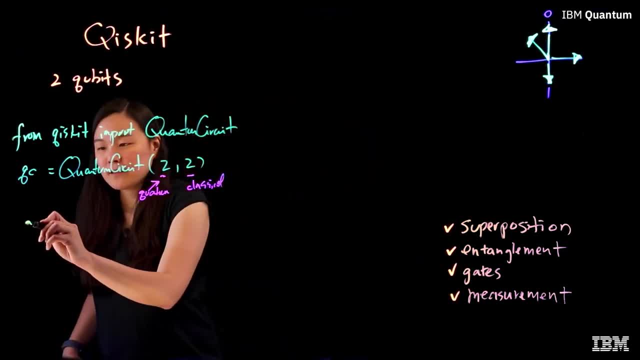 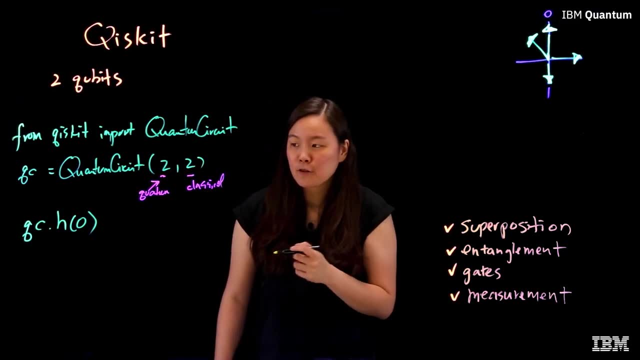 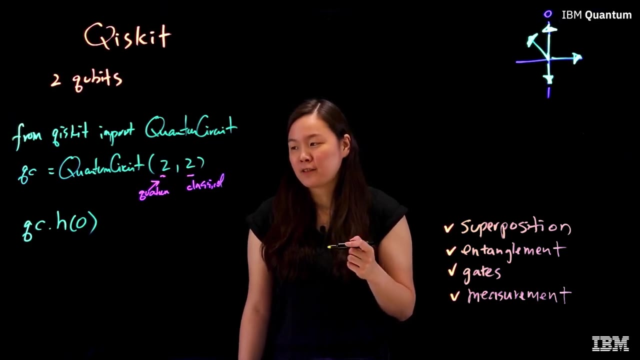 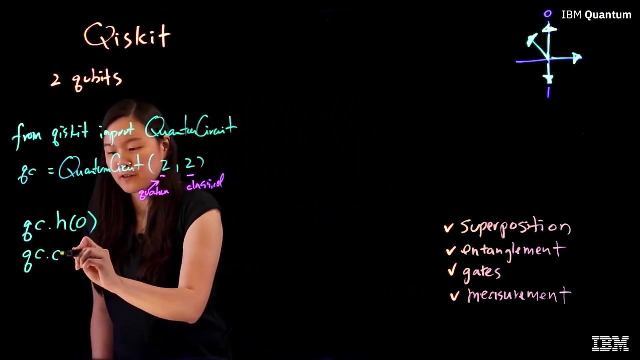 The first one is the Hadamard gate. The Hadamard gate puts the qubit into a superposition between 0 and 1.. That means it now has an equal chance of being measured as 0 or 1.. The next gate we need is the control knot gate, or CX for short. 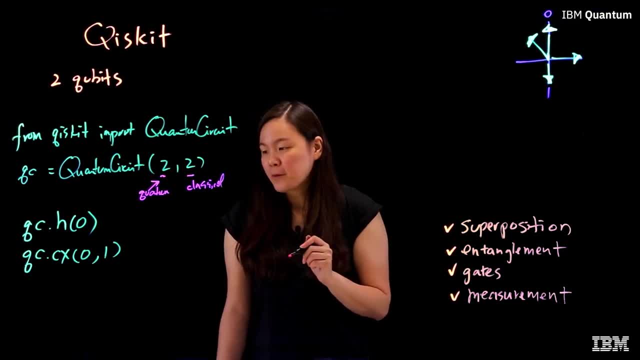 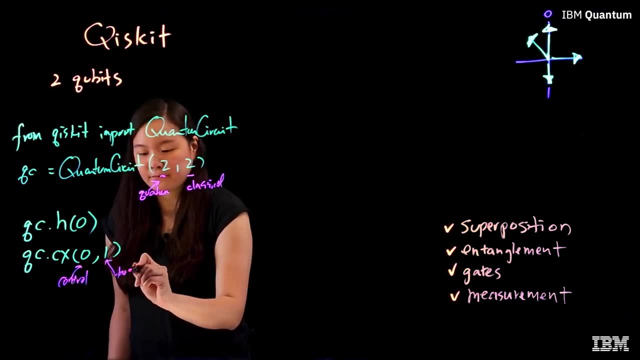 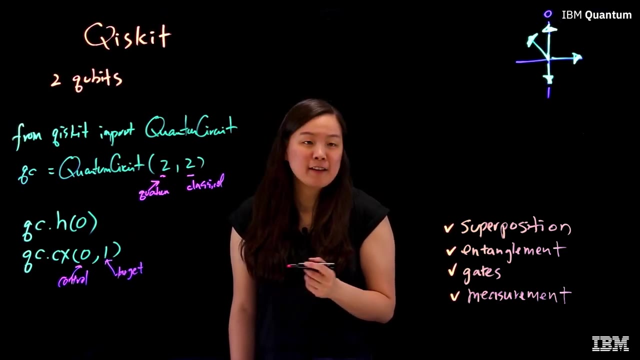 The control knot gate is a conditional two qubit gate. It has a control qubit and a target qubit, Without superposition. the control knot gate is fairly simple to understand, That is it says: if the state of the control qubit is 1, then you flip the state of the. 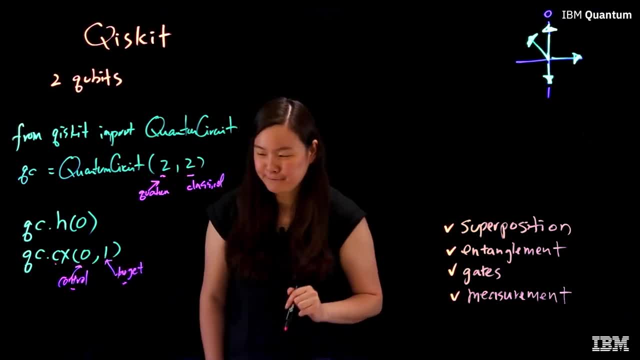 target qubit And that's why it's called a control knot. 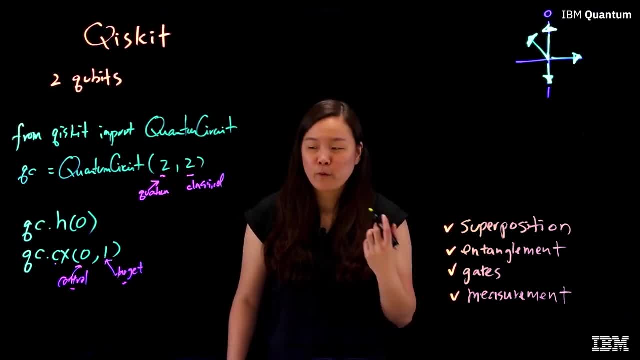 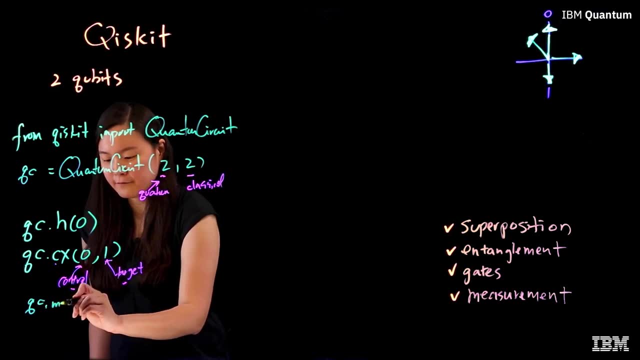 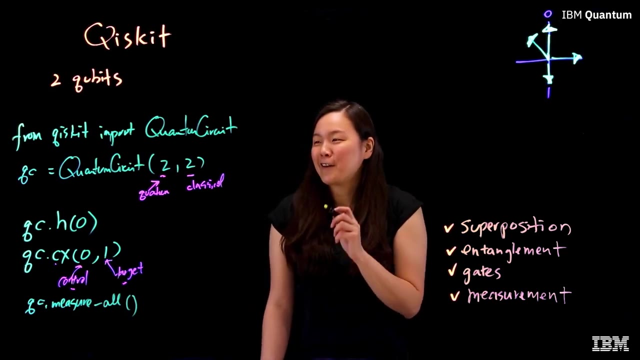 The states of these two qubits are now strongly correlated. We now say they are entangled. So the last thing we want to do is actually do measurements so we can get the outputs, And we do this by calling the measureAll function, And there you have it. 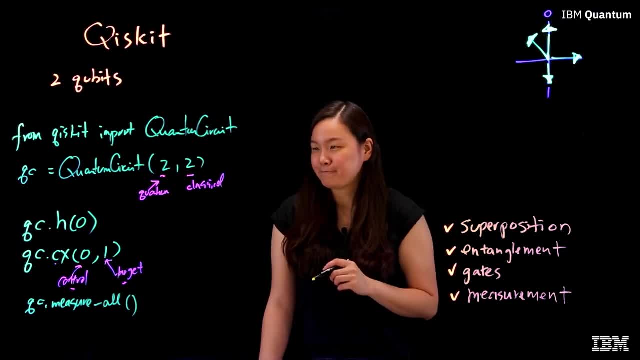 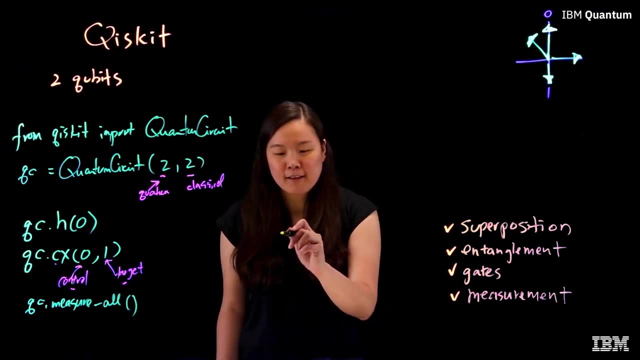 We just wrote a simple quantum program using Qiskit. Now if you take this program and run it a bunch of times on an ideal quantum computer, you'll find out that there is a 50% chance of the output being 0, 0 and 50% chance of 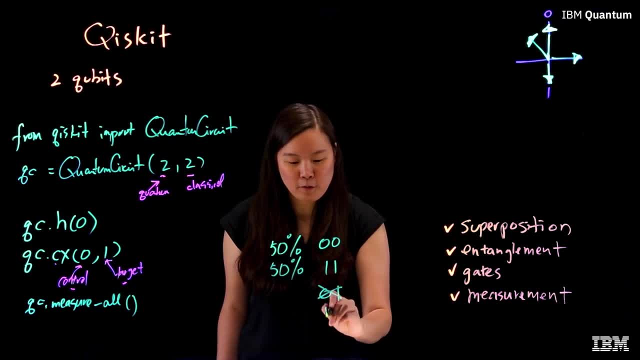 it being 1, 1.. But it would never be a 0, 1 or 1, 0.. The 50, 50 of the first qubits comes from the superposition And while we didn't explicitly change the state of the second qubits, it got changed. 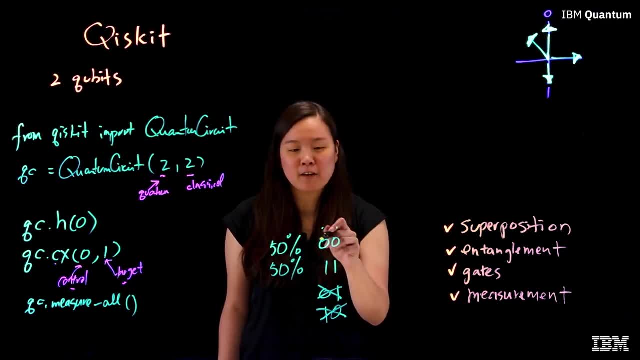 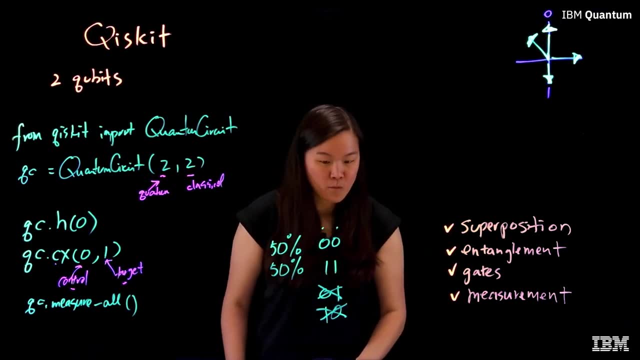 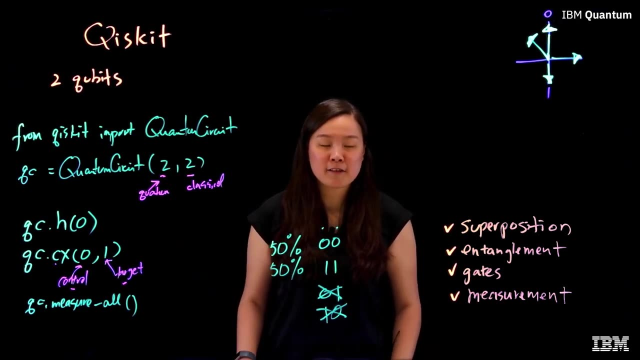 anyway, because it is entangled with the first qubit, So it changes with the first qubit. So in this program we created a quantum circuit which operates at the same level as classical assembly language and allows you to efficiently manipulate the qubits directly. 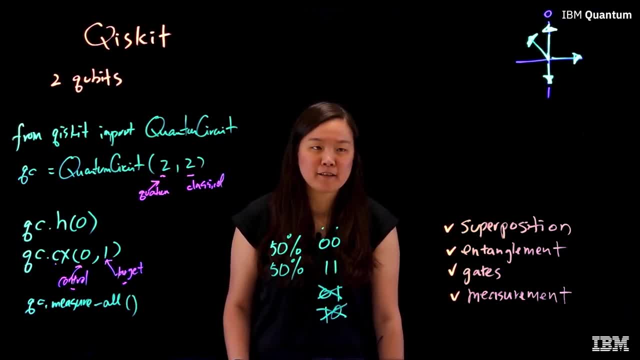 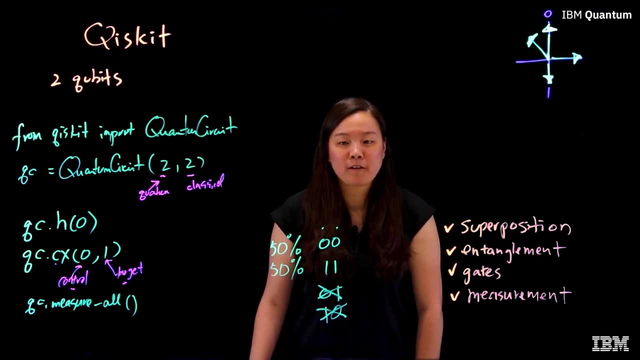 However, if you're not fond of playing with low-level circuits, Qiskit also offers a number of higher-level algorithms. For example, Qiskit has a package called Qiskit Machine Learning that's used for computing quantum circuits, Okay. 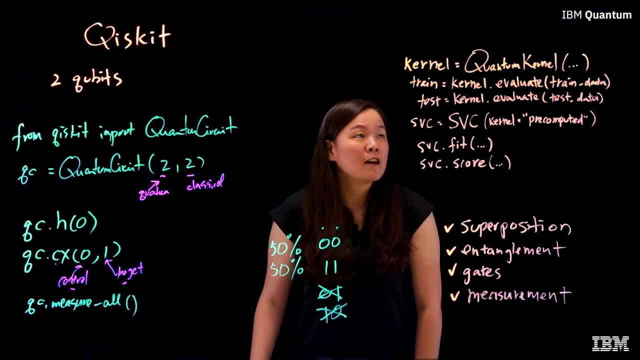 Let's see that has a number of previous classes. You can take a quantum kernel class, use it to train and test data. You can then take this trained quantum kernel and pass it into a classical algorithm such as the support vector classification from scikit-learn.